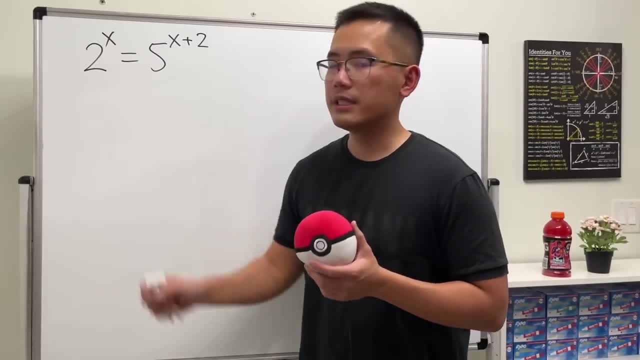 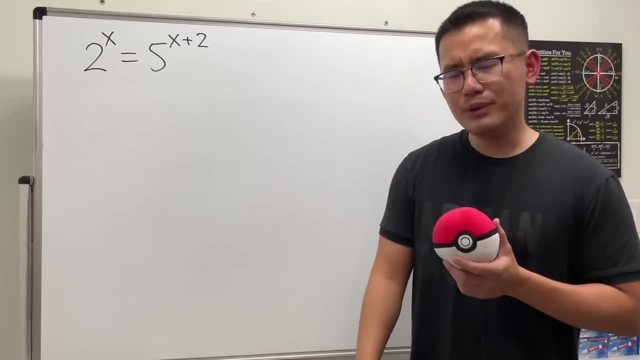 So how do we solve an exponential equation that has two parts and both bases are different? Here we have 2 to the x, that's equal to 5 to the x plus 2. And you know it. please pause the video and try this first. 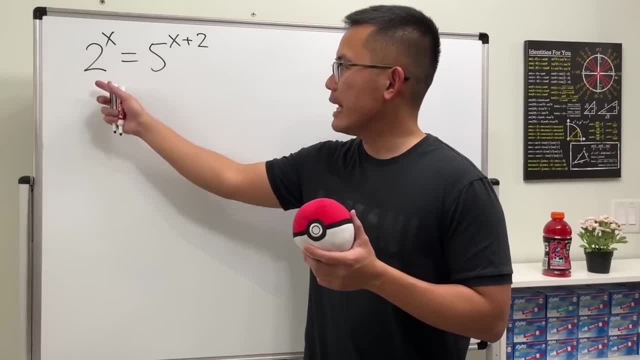 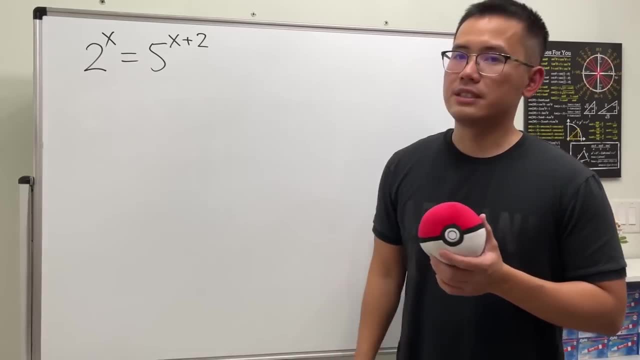 Okay, good, Let's go ahead and continue. The idea is that if we can put exponential parts together on one side, that would be really good. In fact, we can take care of this. Have a look, I'm going to write down 2 to the x, and that's equal to. 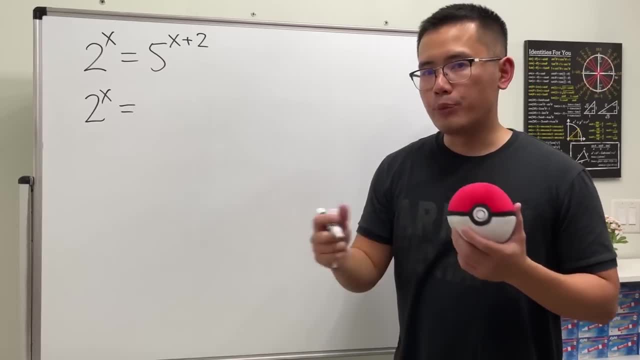 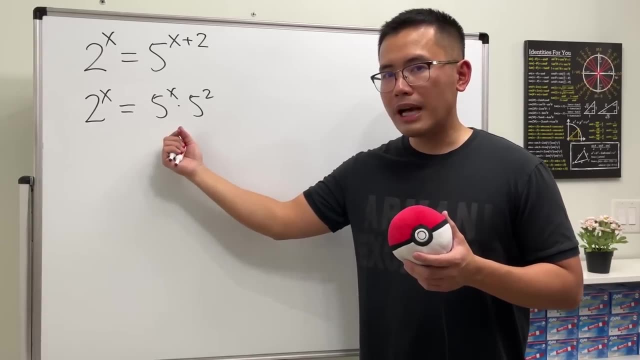 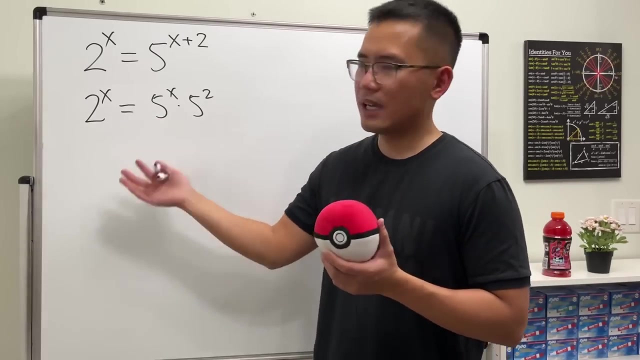 When we have 5 to the x plus 2, we can break them apart as 5 to the x times 5 to the second, Because when they multiply we will just have to add the exponents. Yeah, Good, Now I would like to. just depends on how you want to do it. 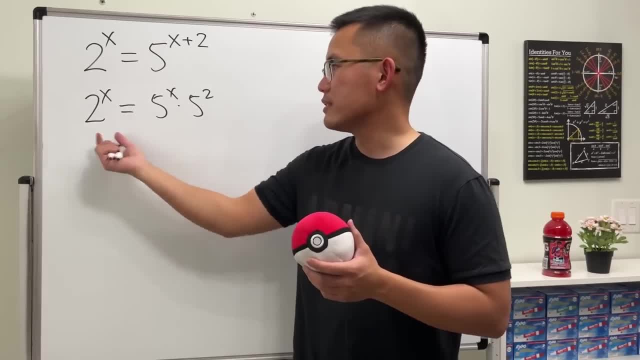 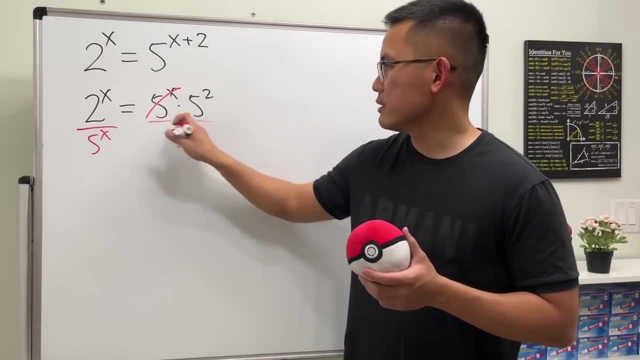 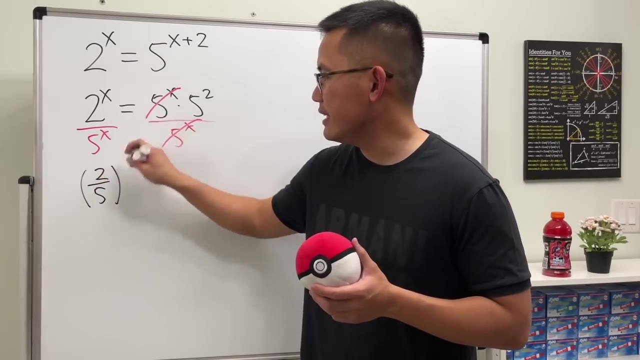 you can divide the 5 to the x on both sides, or you can divide this on both sides, But it would be easier if we do dividing 5 to the x on both sides like this. This way here we will get parentheses with 2 over 5 inside and then the x on the outside. 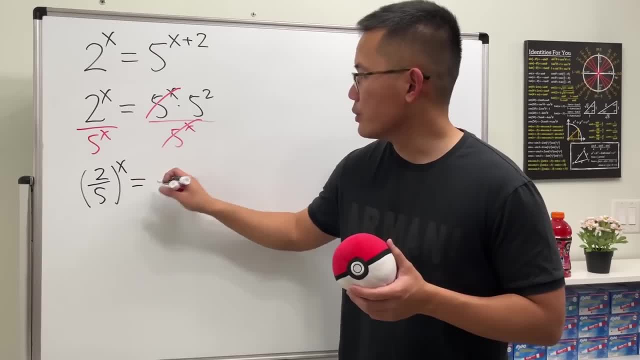 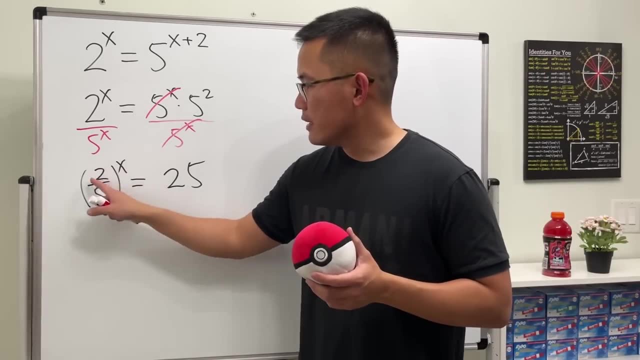 Because they are both with x, And that will be equal to 5 to the second power, and that will be 25.. Now, as you can see, we have some number b raised to the x power, it's equal to 25.. 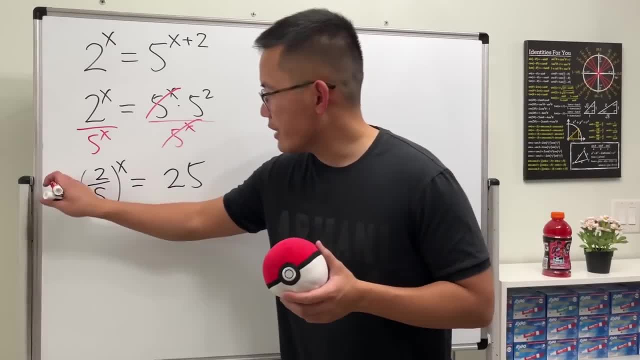 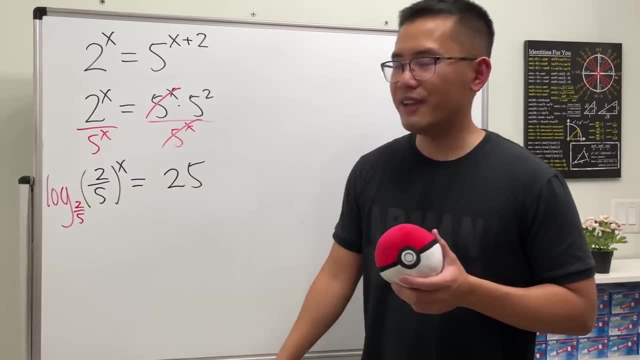 So how do we do this? We take log. Right here we take log, but what base? The same base, Namely 2 over 5.. Right here we do the same thing: Log 2 over 5 for the base. 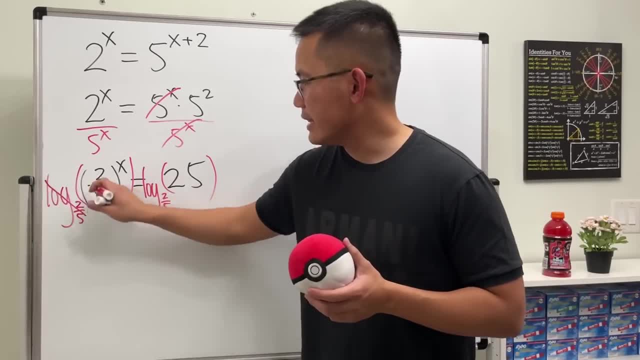 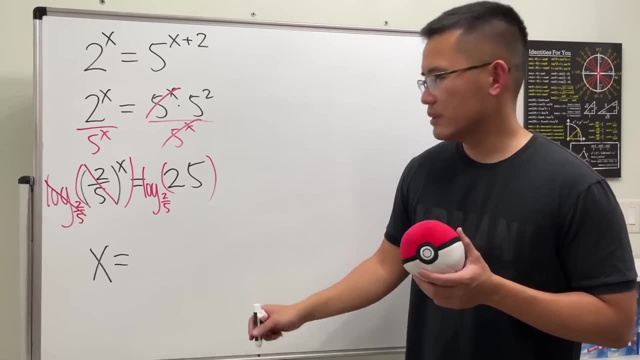 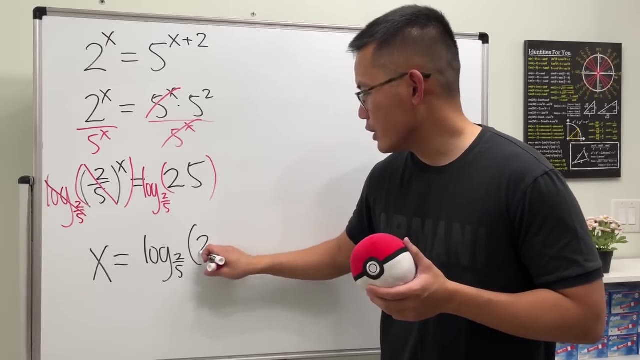 Alright, And on the left-hand side, this and that will cancel, so we just end up with x And that's equal to, and we can just write it down like this. So here I'm going to write this as log base of 2 over 5, and then the input is 25.. 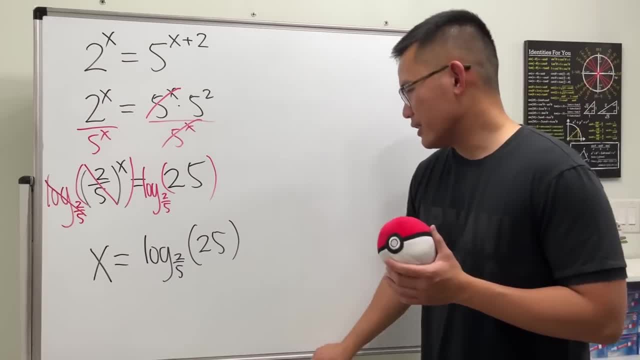 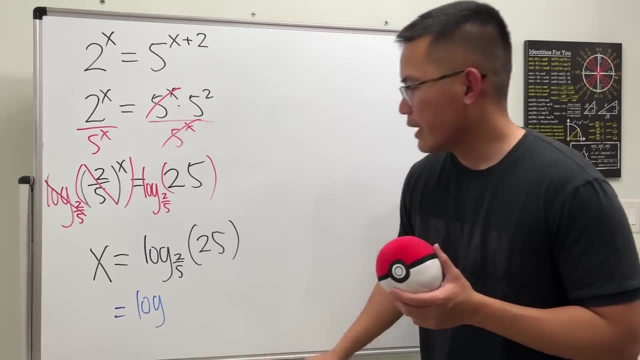 I think this is okay. So to simplify this a little bit, perhaps I will suggest you guys to do the following: This is equal to log, and then we can just do log or ln, up to you, but we can first use the change of base formula.